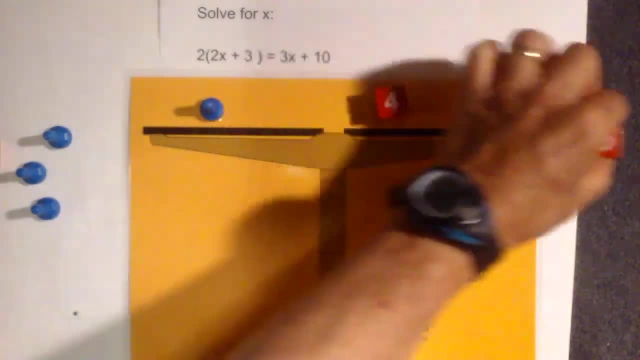 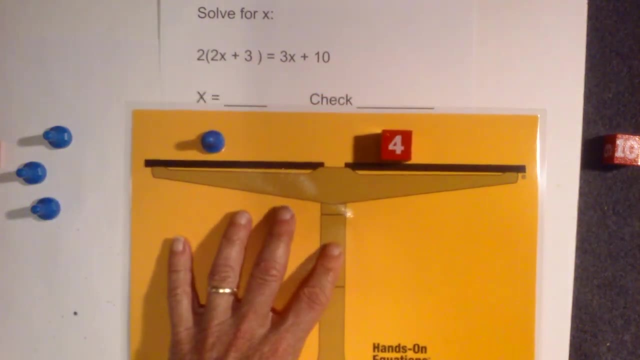 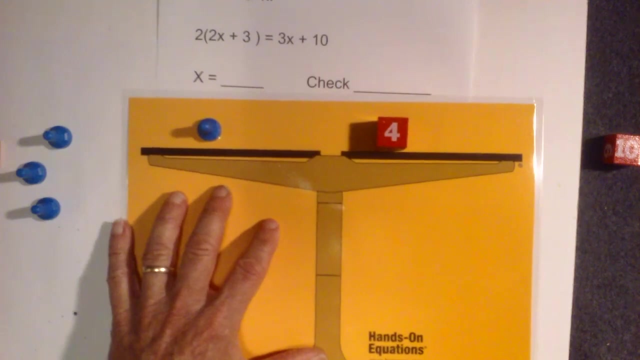 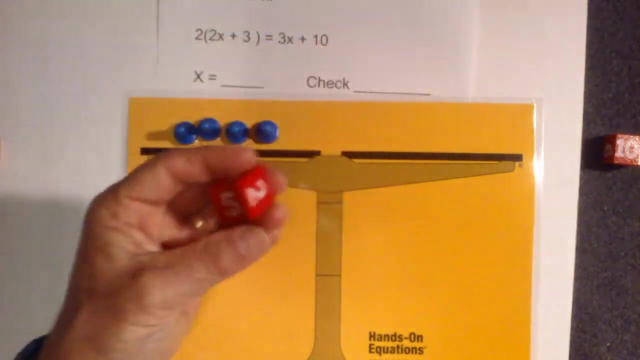 from this side: 10 minus 6 is 4.. Okay, so now I have the answer: x equals 4.. So now I need to check my work. Okay, and so let's check the work. So I need to set my original equation up again. So I have 4x on this side and then I had two 3s. 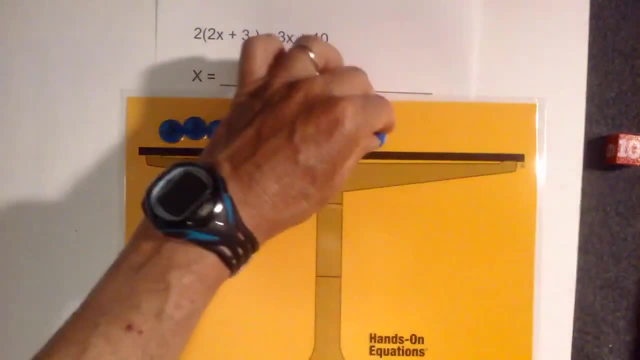 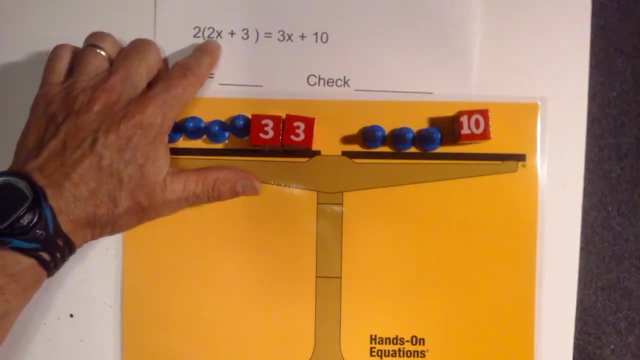 Okay, and then on the other side, we had 3x and 10.. Let's check that. We have 2x plus 3 two times. So there's 2x, 3,, 2x and 3, and then we had 3x and 10.. 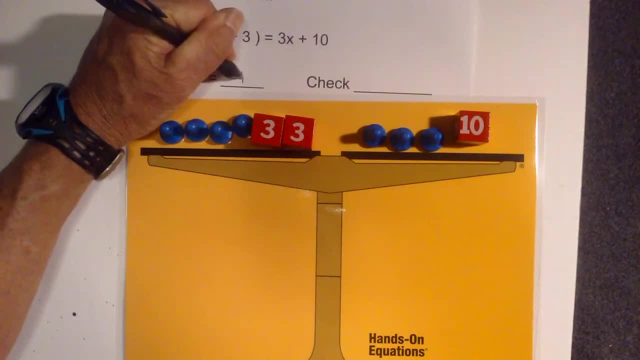 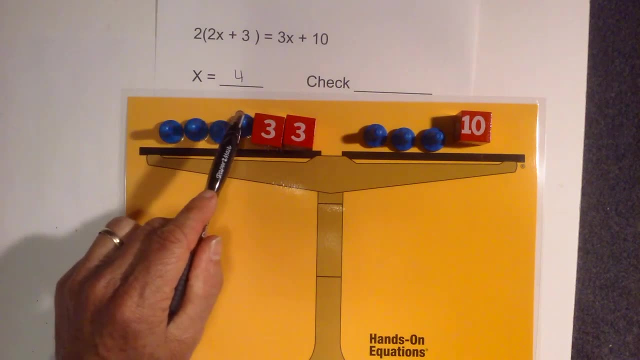 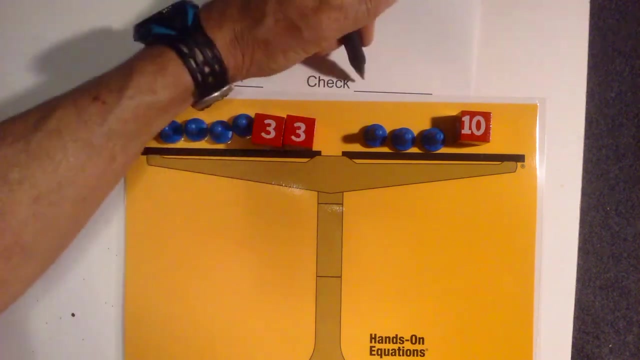 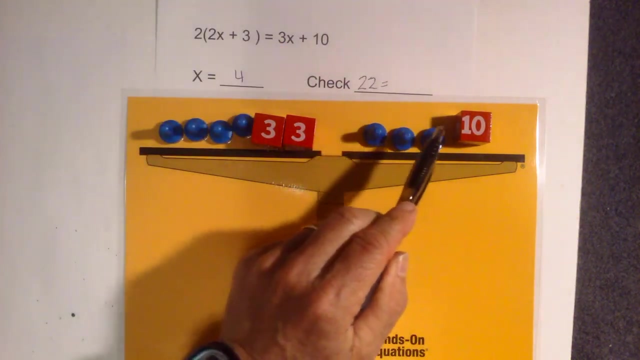 So now I need to check our work and the answer was 4.. So I will go: 4, 8,, 12,, 16,, 17,, 18,, 19,, 20,, 21,, 22.. So I have 22,, and hopefully it will equal 22. on the other side We have 4, 8,, 12 plus 10 is 22.. 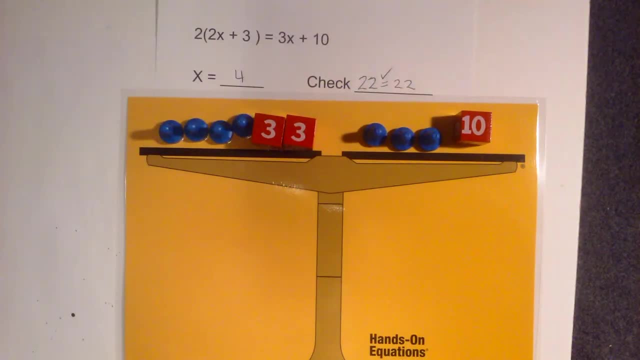 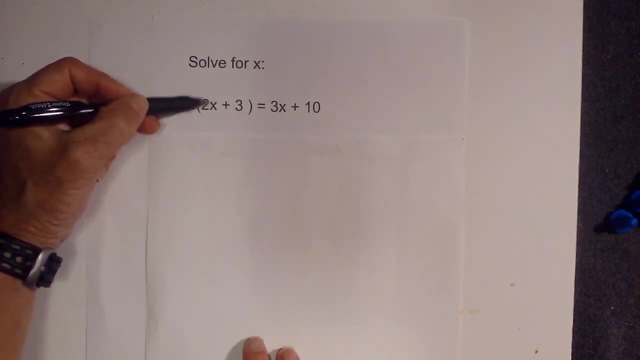 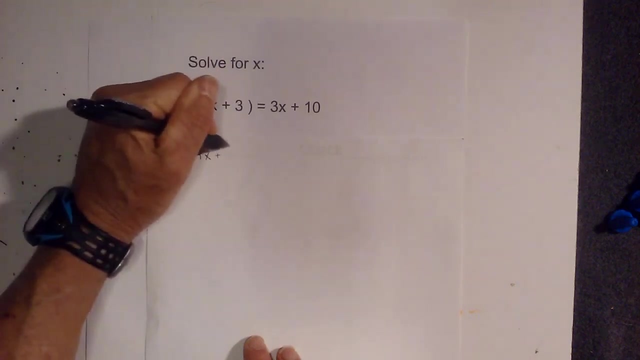 It works. Now let's solve this the traditional way. And solve this the traditional way. The number on the outside means you multiply by what's on the inside. 2 times 2x is 4x. 2 times 3 is 6, equals 3x plus 10.. And if you remember, 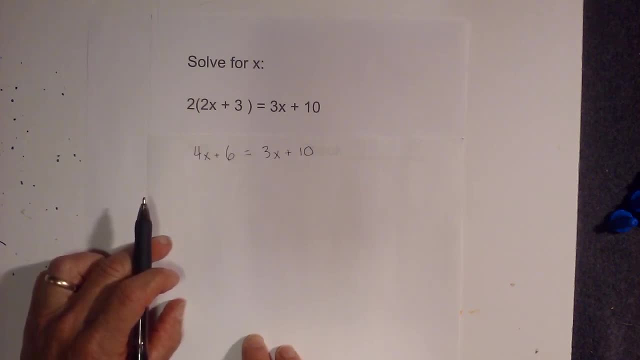 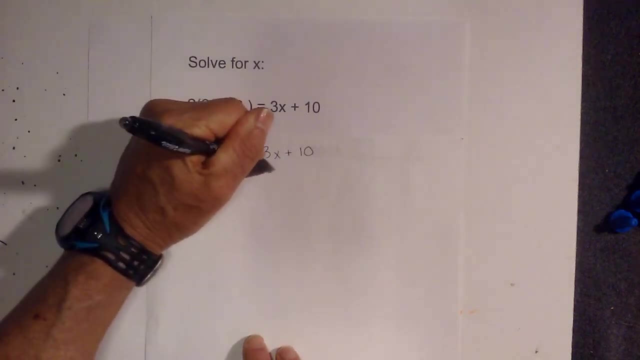 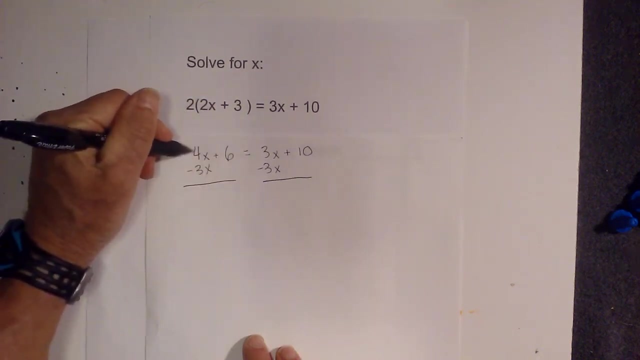 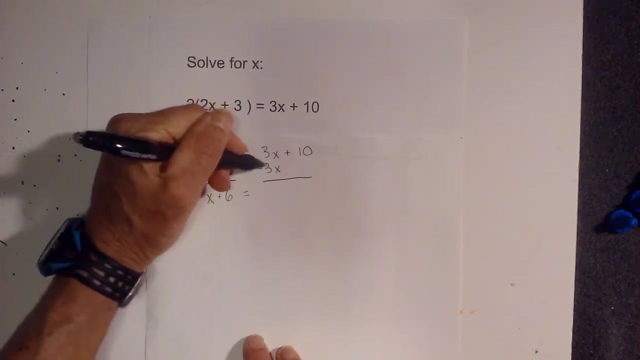 that's exactly what we had when we had our physical setup, So I can subtract x's from each side and I can remove 3.. So now I have 3x Subtract, 3x there and 3x here. When I subtract 4 minus 3x equals x, I'm going to bring down the 6 equals 3 minus 3 is. 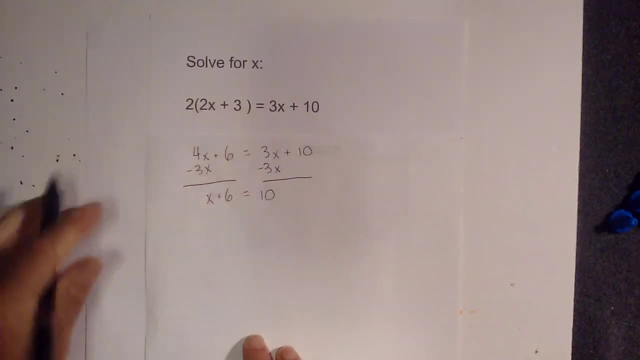 0. So they cancel. So I'm going to bring down the 10.. Now I can remove numbers, So I'm going to subtract 6 from each side And bring down the x. 6 minus 6 is 0 equals 4.. So the answer is 4.. And now I'm going to check my work.